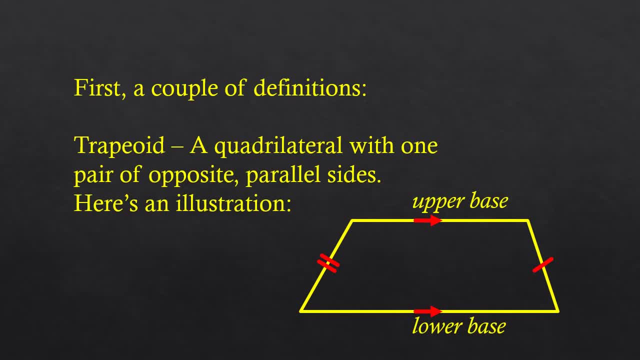 two sides are not necessarily equal in length. They're not necessarily congruent, as we say, And uh. so that's why I have one tick mark on one side and two tick marks on the other side, And these non-parallel sides of a trapezoid are called the legs of the trapezoid. 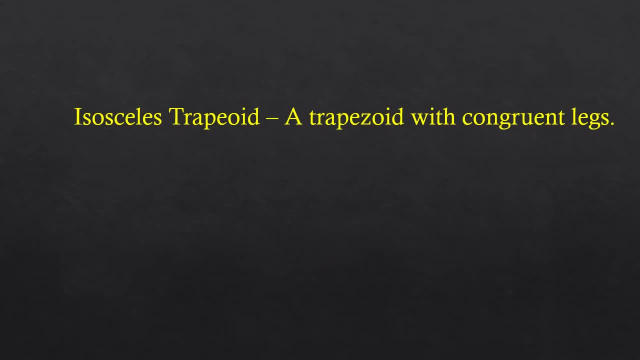 And one other definition is that an isosceles trapezoid is a trapezoid with congruent legs. just like an isosceles triangle is a triangle with two congruent sides, An isosceles trapezoid is a trapezoid with congruent legs. That might look something. 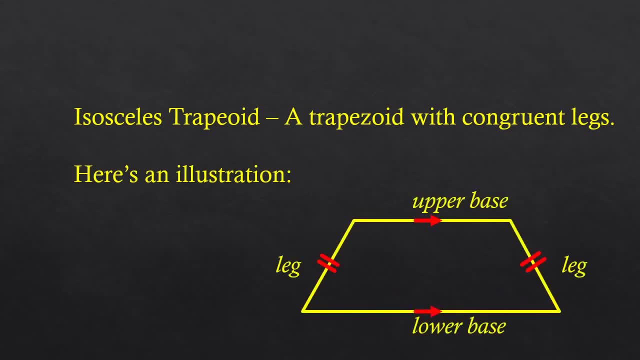 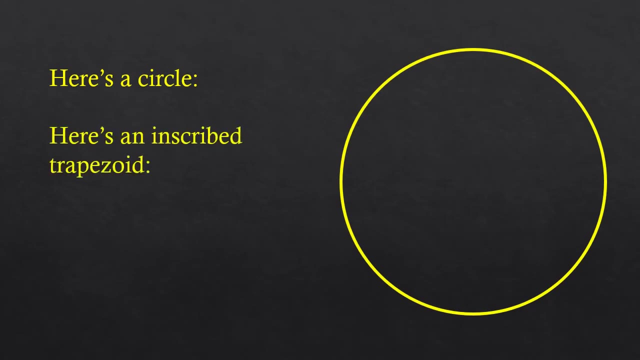 like this: You have the upper and lower base that are parallel to each other, but now the legs are of the same length. In other words, they're congruent. So let's take a circle and let's inscribe a trapezoid into it. Now to inscribe a polyphonic 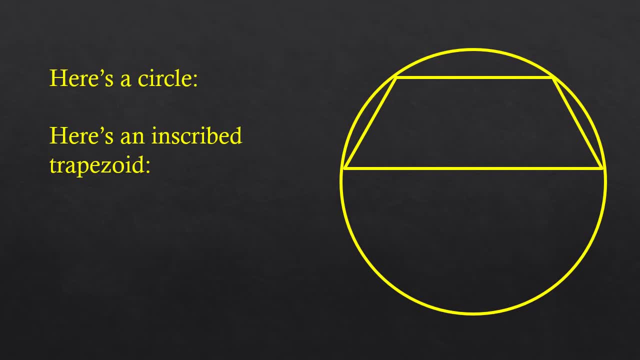 polygon into a circle means that the points of the polygon are touching the circle on the inside. So here are the trapezoid. the four points of the trapezoid, the four vertices of the trapezoid are touching the circle. 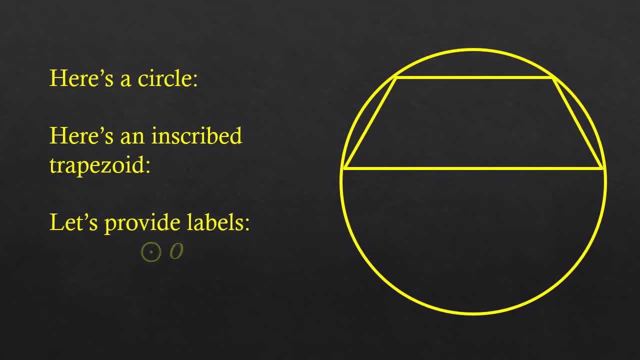 And let's put some labels on this so we can talk about it. The circle we'll call circle O, So there's the center of the circle, and we'll call that point O. That defines the circle. It has a particular radius. And then the trapezoid we'll label ABCD, like that. 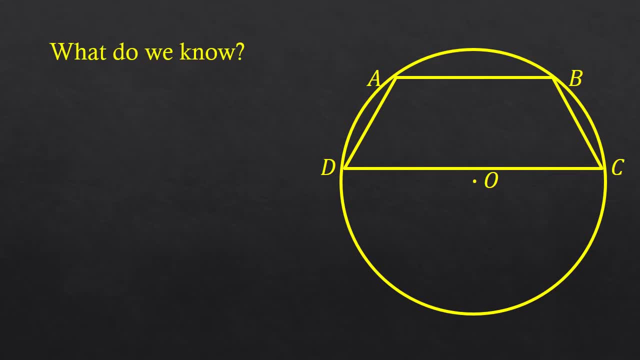 Okay. so what do we know about this picture? So we're given this picture. We know that it's a trapezoid. We know that, since it is a trapezoid, the bases must be parallel. That's one of the parts or the definitions of the trapezoid. That means that in the trapezoid, the trapezoids are parallel to each other. That means that in the trapezoid, the trapezoids are parallel to each other. That means that in the trapezoid, 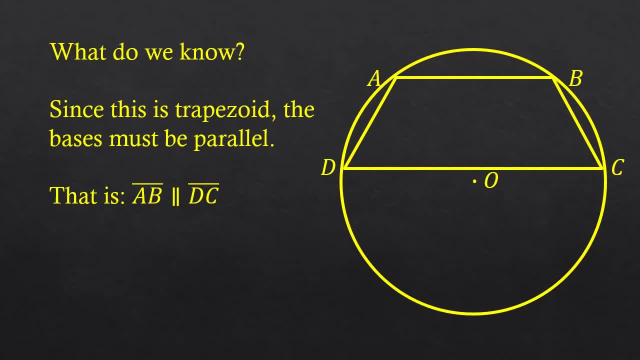 in this picture, AB is parallel to DC. So how do we approach the problem? Of course, this is the key question when doing a geometric proof: Where do we go from here? Okay, so, in this problem, what I'm going to do is I'm 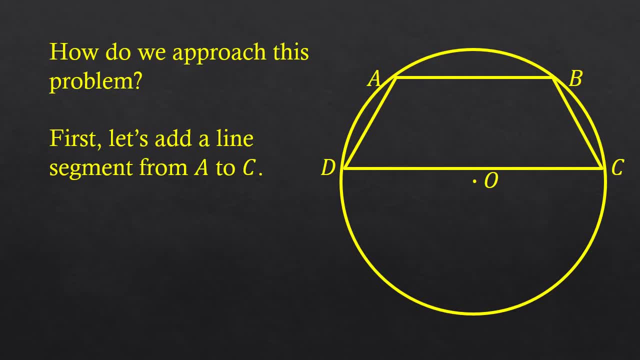 going to draw a line segment from A to C. You can always draw line segments on a figure to help prove this. So here in this blue line I've drawn is from A to C. Now, since AB and DC are parallel to one another, we can consider that this AC is a transversal. And since we know that, 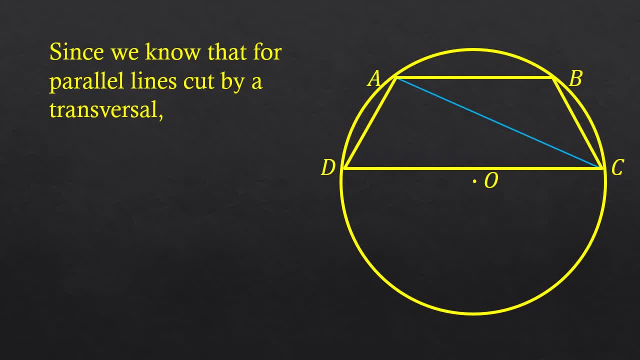 for parallel lines cut by such a transversal, the alternate interior angles are congruent, That is, angle ACD is congruent to angle CAB, And those are shown here in red. Now, the other thing about this picture is that the two angles that are shown there 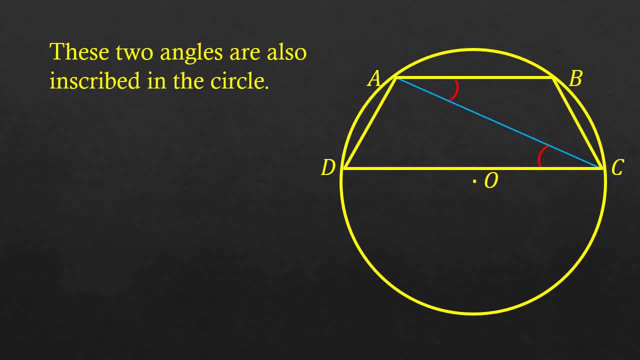 ACD and CAB are inscribed angles. That means that their vertices are on the circle and they cut out a particular arc. Now, one property of these is: if the inscribed angles are congruent, then the subtended arcs that they cut out are also congruent. 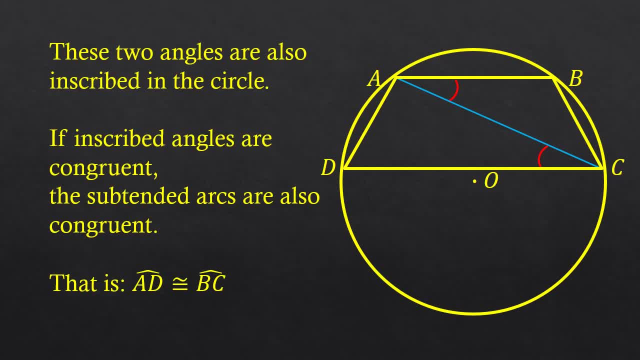 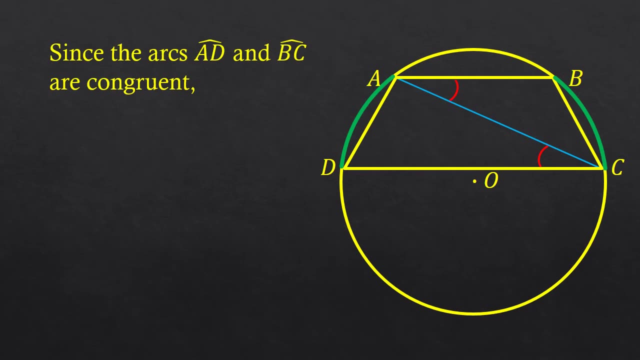 That is, arc AD is congruent to arc BC. That means that their angular measure is the same. So if the inscribed angles are congruent, then the subtended arcs that they cut out are also congruent Now, and they're shown there in green. 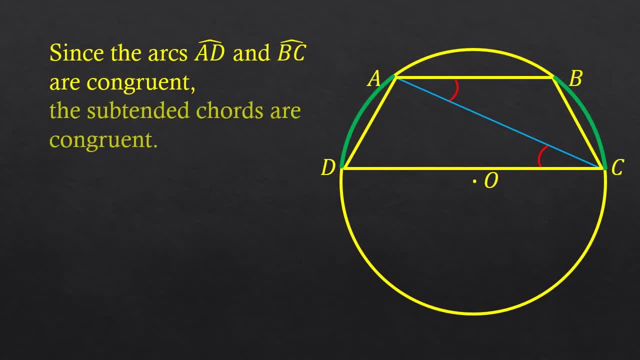 Since these arcs are congruent, the subtended cords are also congruent, That is, line segment AD and line segment BC are congruent to one another, And they're shown there in red. Well, if that's true, then note that these are also the legs of the trapezoid, And therefore 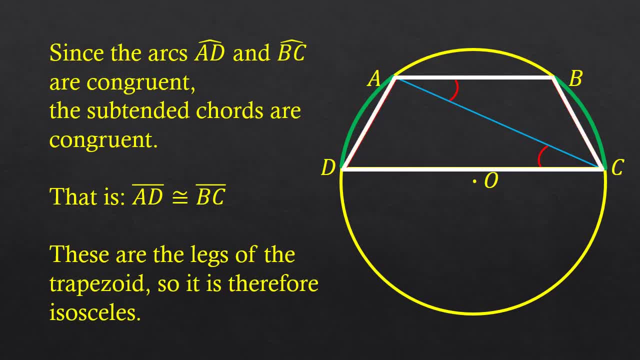 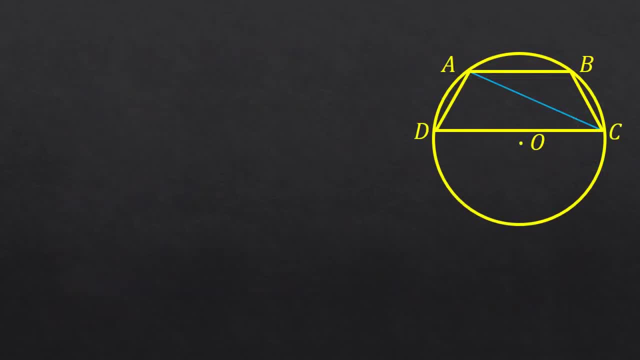 the trapezoid itself must be an isosceles trapezoid. So now let's put the. once we have all of the steps, we can organize them into a table in the statement reason form that we are familiar with. 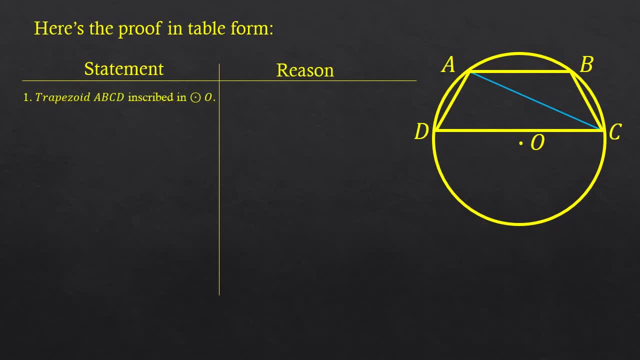 So the first thing we're going to do is we're going to take the first step, and we're going to take the second step, and we're going to take the third step, and we're going to take the fourth step. The first statement is this: 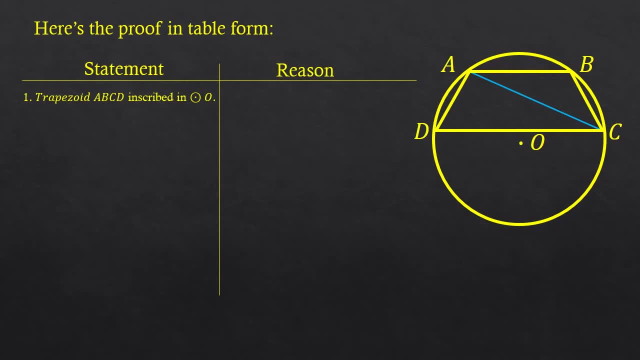 The trapezoid ABCD is inscribed in circle O. The reason for that is: well, that's the given information. That's what we're starting with. Statement number two: draw segment AC. The reason for this is often given as construction. 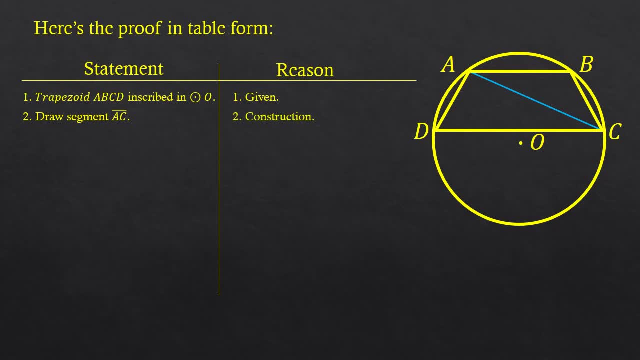 We can do that for any figure. We can draw additional auxiliary lines. The third step is that segment AB is parallel to DC. Now, the reason for that is that this is a property of the trapezoid, that the bases of a trapezoid are parallel to one another. 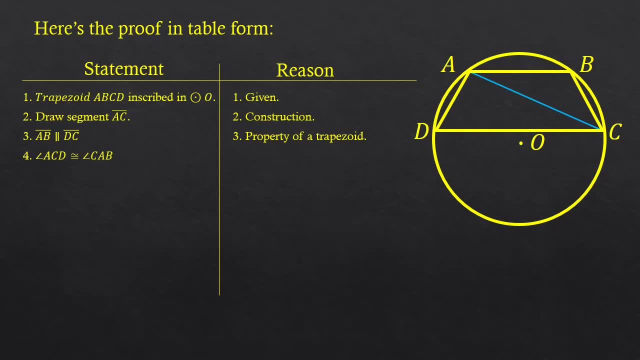 The fourth step is that triangle, ACD and angle- excuse me, angle ACD is parallel to. let me start over. Angle ACD is congruent to angle CAB And the reason for that is that these are alternate interior angles of parallel lines. 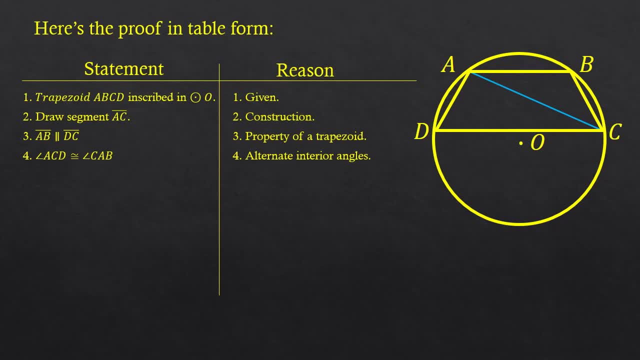 cut by a transversal. Step five is that ACD, angle ACD and angle CAB are inscribed angles. Okay, And the reason is that their vertices and endpoints lie on the circle. So knowing that arc AD is congruent to arc BC because congruent inscribed angles create